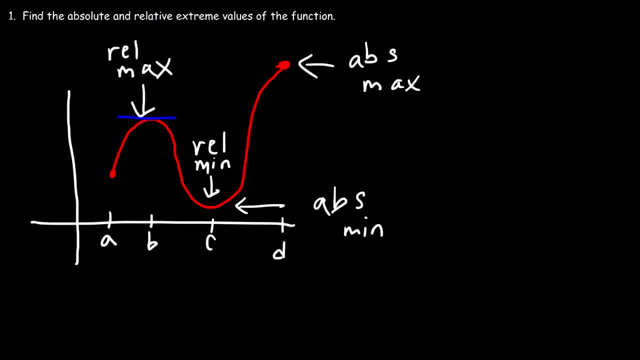 To identify the relative extrema, you need to identify the locations where the slope is zero. Since we have a horizontal tangent line, the slope will be equal to zero And the slope will be equal to zero, So you need to use the first. 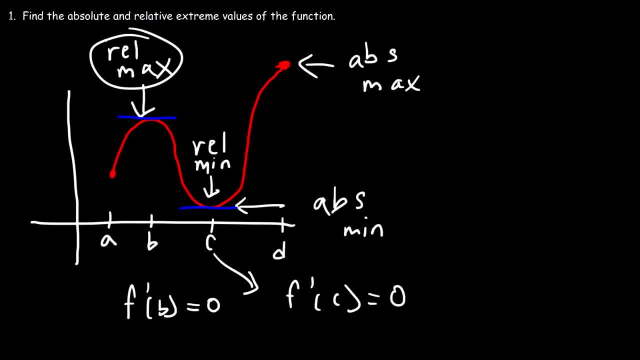 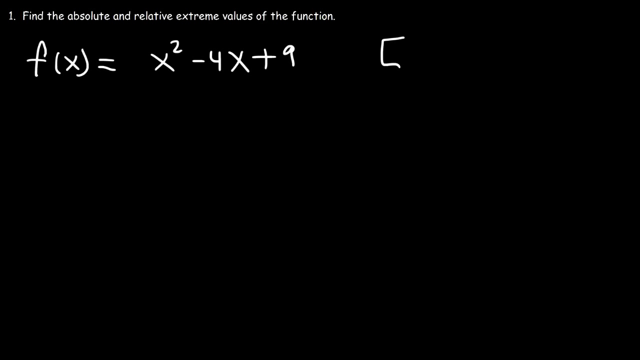 derivative to find the location of any relative extrema. Now let's work on a practice problem. So let's say that f of x is equal to x squared minus 4x plus 9. And identify any absolute and relative extreme values of the function anywhere in the interval between 1 and 4.. 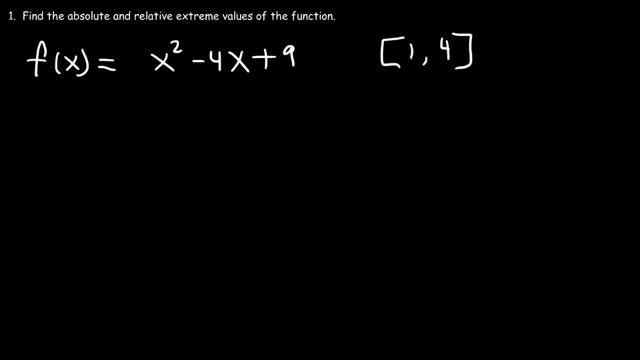 So the first thing I would recommend doing is identifying the critical points, That's where the first derivative is equal to zero. At those locations you could find any relative extreme values, like a relative min or max. The derivative of x squared is 2x. The derivative of negative 4x is negative 4x. 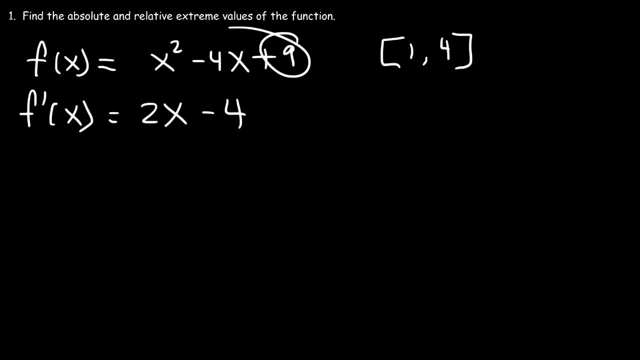 And the derivative of a constant is zero. So let's set this equal to zero. Now let's take out a 2.. So this is going to be x minus 2.. If we divide both sides by 2,, 0 is equal to x minus 2.. And if we add 2,, x is equal to 2.. So we have 2 as the critical number. 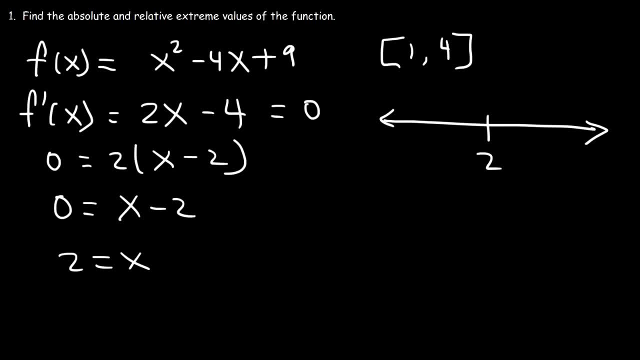 And we need to identify if this is going to be a relative maximum or a relative minimum. So we need to create a sign chart. So let's make a number line. Now we need to determine what the slope is going to be to the left and to the right of 2.. 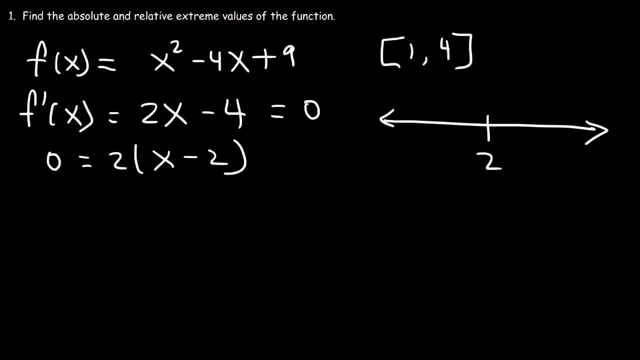 So let's pick a number that's greater than 2.. Let's try 3.. If we plug in 3 into the first derivative, 3 minus 2 is positive, So the result will be positive. If we plug in a number that's less than 2, like 1, into the first derivative, 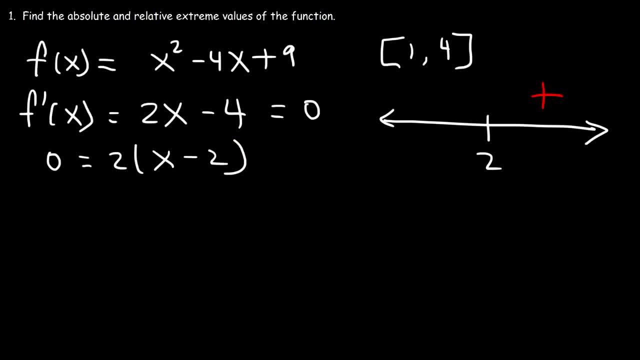 1 minus 2 will be negative, And then if we multiply that by 2, that will give you a negative result. So notice that the slope changes from negative to positive across the critical point. So at 2, do we have a relative maximum or a relative minimum? 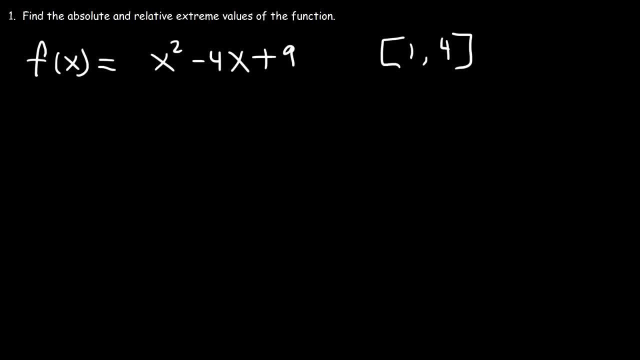 So the first thing I would recommend doing is identifying the critical points, That's where the first derivative is equal to zero. At those locations you could find any relative extreme values, like a relative min or max. The derivative of x squared is 2x. The derivative of negative 4x is negative 4x. 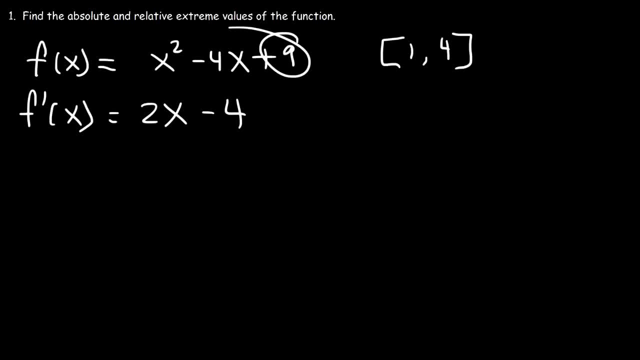 And the derivative of a constant is zero. So let's set this equal to zero. Now let's take out a 2.. So this is going to be x minus 2.. If we divide both sides by 2,, 0 is equal to x minus 2.. And if we add 2,, x is equal to 2.. 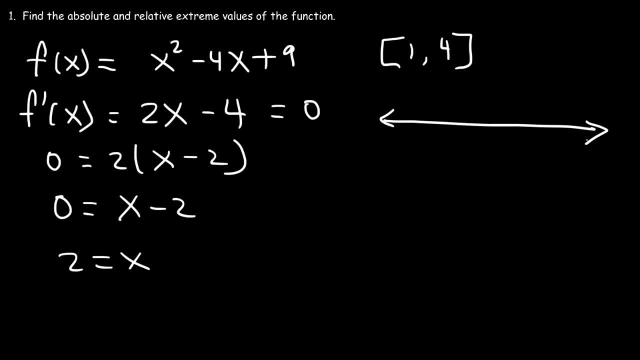 So we have 2 as the critical number And we need to identify if this is going to be a relative maximum or a relative minimum. So we need to create a sine chart. So let's make a number line. Now we need to determine what the slope is going to be to the left and to the right of 2.. 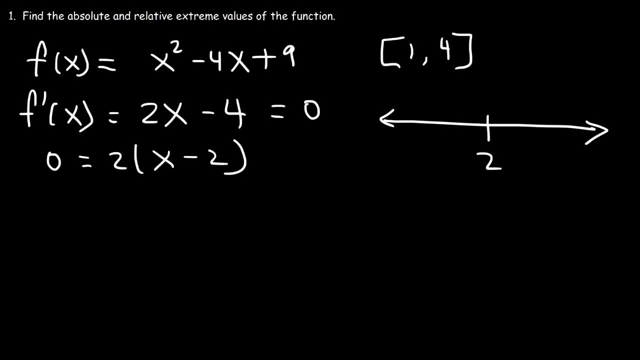 So let's pick a number that's greater than 2.. Let's try 3.. If we plug in 3 into the first derivative, 3 minus 2 is positive, So the result will be positive. If we plug in a number that's less than 2, like 1, into the first derivative, 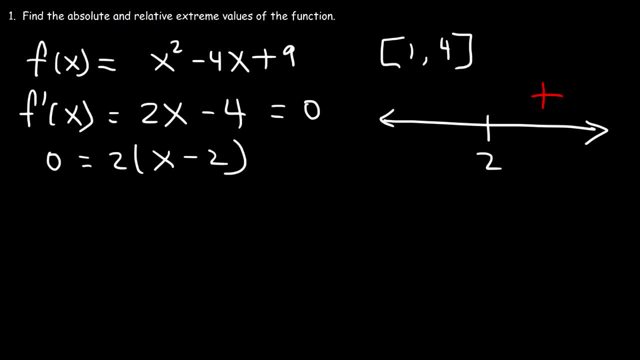 1 minus 2 will be negative, And then if we multiply that by 2, that will give you a negative result. So notice that the slope changes from negative to positive across the critical point. So at 2, do we have a relative maximum or a relative minimum? 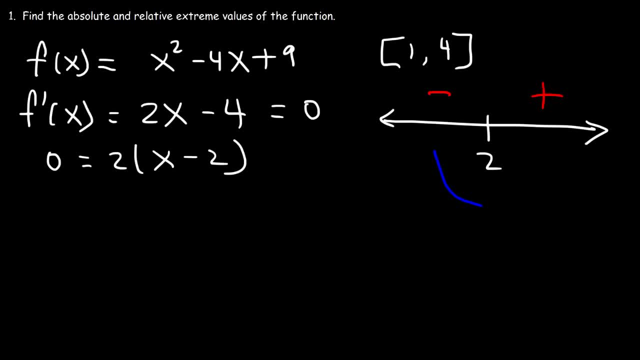 When a slope is negative, the function is decreasing, And when it's positive, the function is increasing, And so this is a minimum. So we have a relative minimum at x equals 2.. So now let's move on to the absolute extreme values. 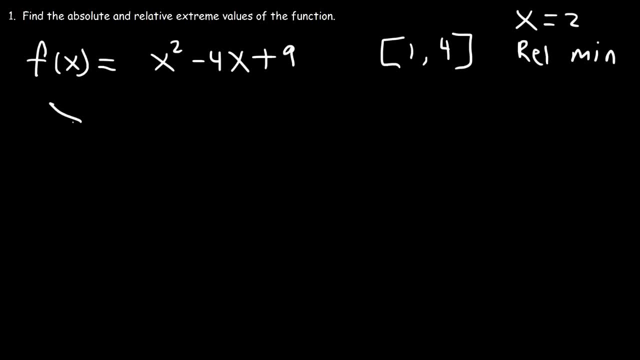 So once you have all of the critical points, make a table. Now on the table you want to put the endpoints of the interval, so 1 and 4. And then in between that any critical numbers that you have. Now we need to determine the slope. 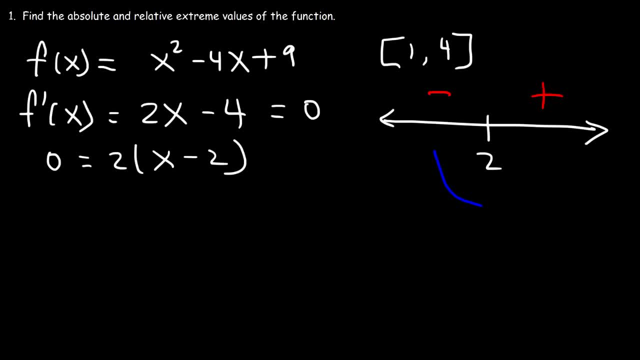 When a slope is negative, the function is decreasing, And when it's positive, the function is increasing, And so this is a minimum. So we have a relative minimum at x equals 2.. So now let's move on to the absolute extreme values. 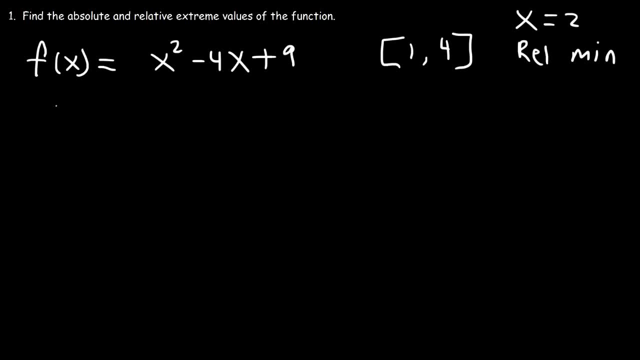 So once you have all of the critical points, make a table. Now on the table you want to put the endpoints of the interval, So 1 and 4. And then in between that any critical numbers that you have. Now we need to determine what the slope is. 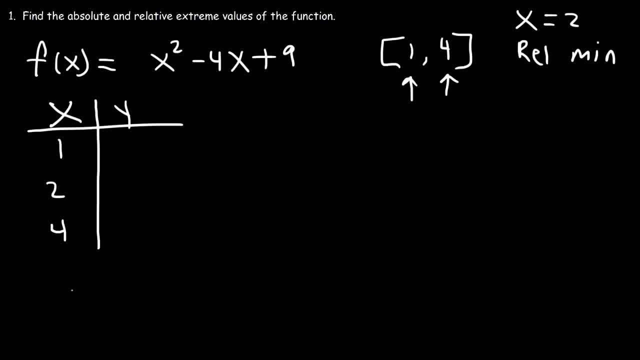 We need to determine the y values for each of these x values. So we need to plug in the values into this function to get y. So let's start with 1.. f of 1 is going to be 1 squared minus 4 times 1 plus 9.. 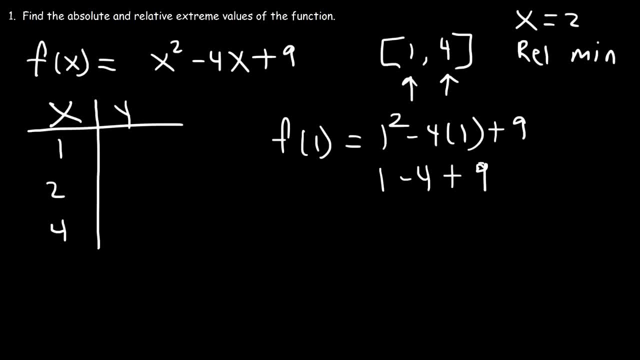 So this is 1 minus 4 plus 9.. 1 plus 9 is 10.. 10 minus 4 is 6.. So f of 1 is equal to 6.. Now let's evaluate the function when x is 2.. 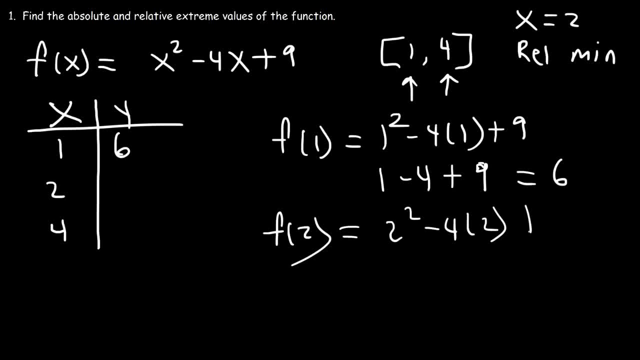 So this is 2 squared minus 4 times 2 plus 9.. 2 squared is 4.. 4 times 2 is 8.. 4 minus 8 is negative, 4.. Negative: 4 plus 9 is 5.. 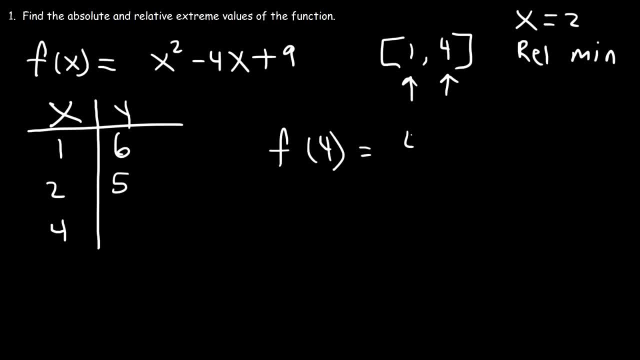 Now let's evaluate the function when x is 4.. 4 squared is 16.. 4 times 4 is the same thing: 16 minus 16 is 0.. 0 plus 9 is 9.. So f of 4 is equal to 9.. 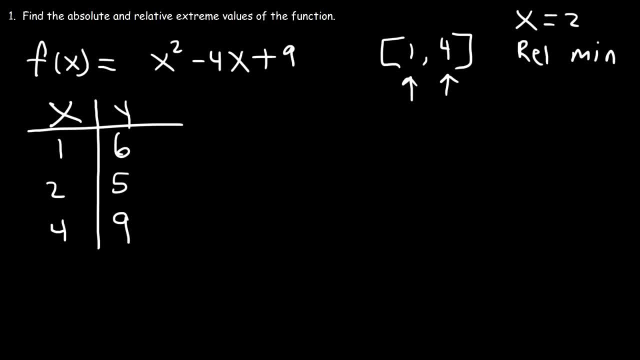 So notice that 9 is the highest y value. Therefore, 9 is the absolute maximum value of the function. 5 is the absolute minimum value Because 5 is less than 6 and 9.. In addition, it's also the relative minimum. 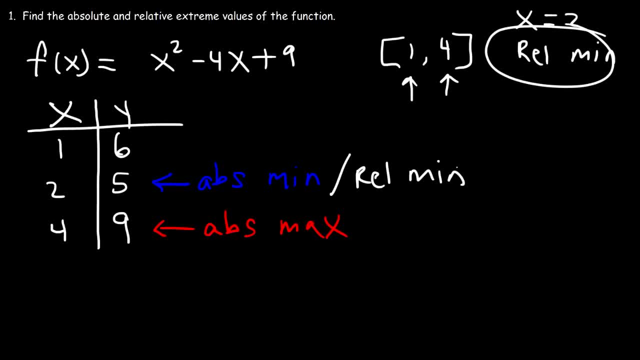 So it's both the absolute minimum and the relative minimum on the interval of 1 to 4.. And so that's how you could find the absolute extreme values of the function as well as the relative extreme values. Now let's work on another problem. 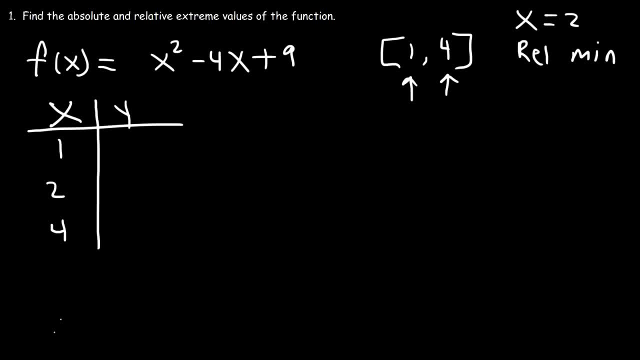 We need to determine the y-values for each of these x-values, So we need to plug in the values into this function to get y. So let's start with 1.. f of 1 is going to be 1 squared minus 4 times 1 plus 9.. 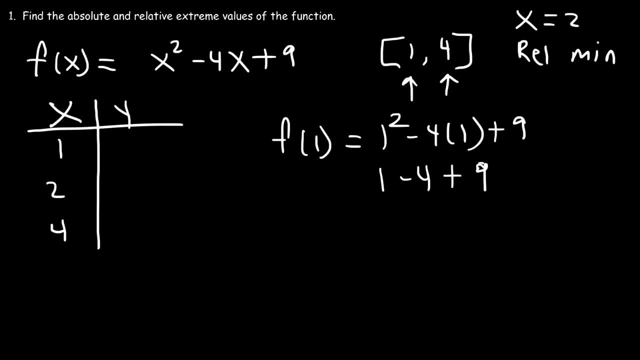 So this is 1 minus 4 plus 9.. 1 plus 9 is 10.. 10 minus 4 is 6.. So f of 1 is equal to 6.. Now let's evaluate the function when x is 2.. 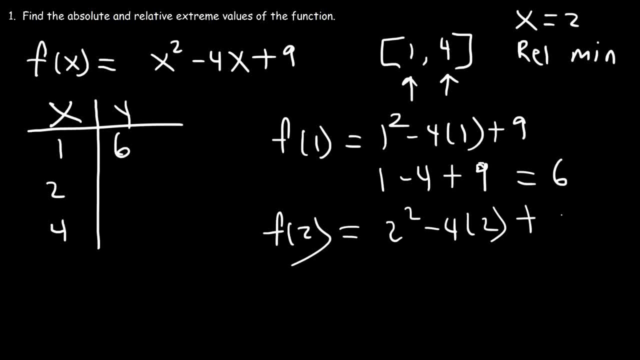 So this is 2 squared minus 4 times 2 plus 9.. 2 squared is 4.. 4 times 2 is 8.. 4 minus 8 is negative, 4.. Negative: 4 plus 9 is 5.. 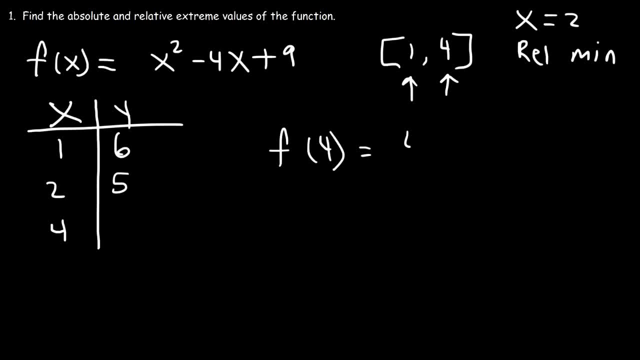 Now let's evaluate the function when x is 4.. 4 squared is 16.. 4 times 4 is the same thing: 16 minus 16 is 0.. 0 plus 9 is 9.. So f of 4 is equal to 9.. 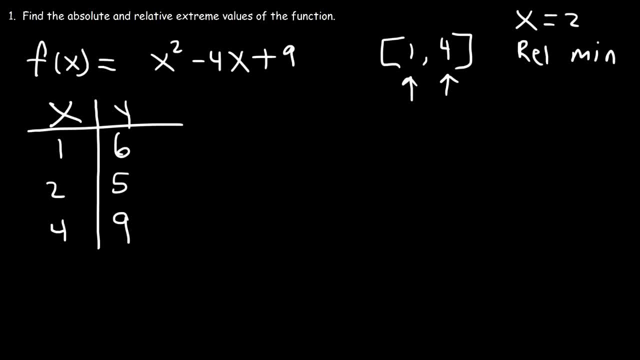 So notice that 9 is the highest y-value. Therefore, 9 is the absolute maximum value of the function. 5 is the absolute minimum value Because 5 is less than 6 and 9.. In addition, it's also the relative minimum. 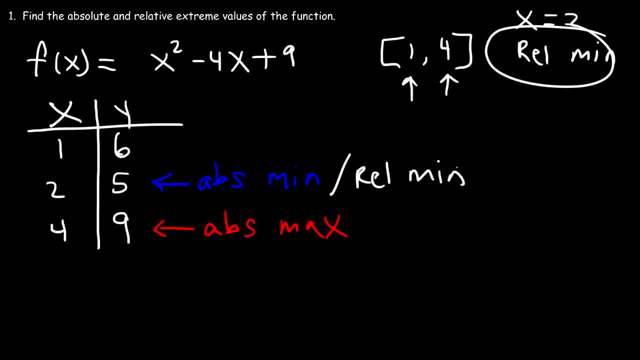 So it's both the absolute minimum and the relative minimum on the interval of 1 to 4.. And so that's how you could find the absolute extreme values of the function as well as the relative extreme values. Now let's work on another problem. 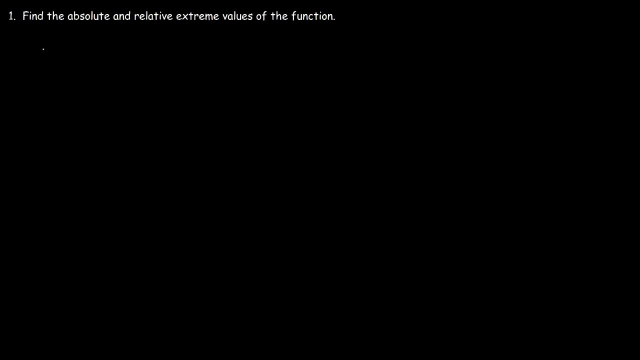 So let's use a different function. So f of x will be equal to, let's say, 4x cubed minus 39x squared plus 90x plus 2.. So identify all of the absolute and relative extreme values of the function on the interval 1 to 6.. 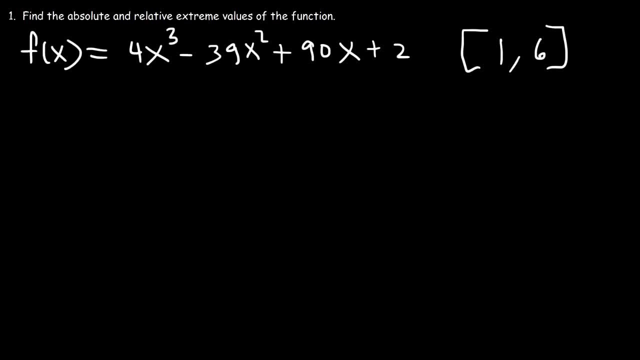 So feel free to pause the video if you want to try this problem. So let's begin by finding the critical numbers of the function. So we need to find the first derivative. in order to do that, The derivative of x cubed is 3x squared. 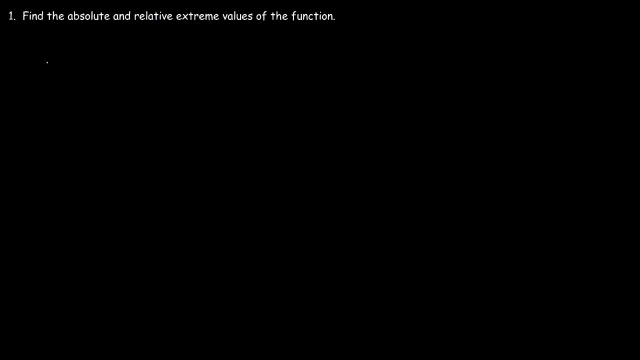 So let's use a different function. So f of x will be equal to, let's say, 4x cubed minus 39x squared plus 90x plus 2.. So identify all of the absolute and relative extreme values of the function. 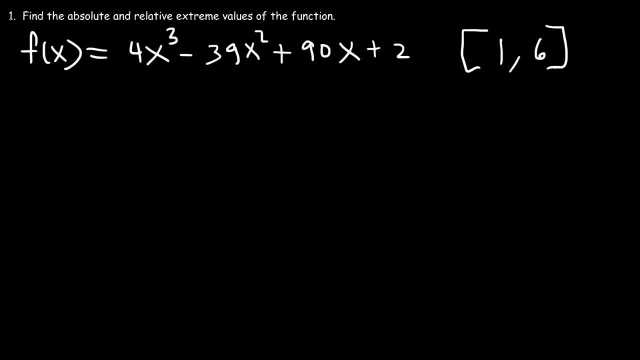 on the interval 1 to 6.. So feel free to pause the video if you want to try this problem. So let's begin by finding the critical numbers of the function. So we need to find the first derivative in order to do that. 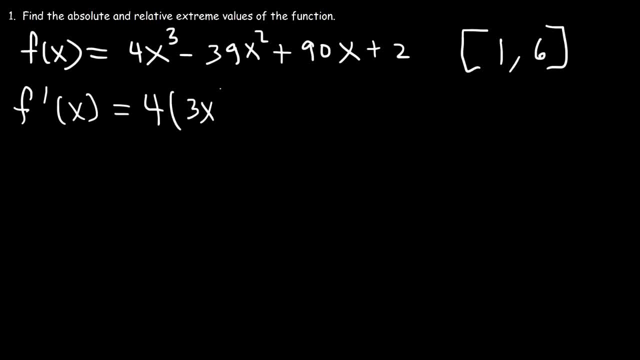 The derivative of x cubed is 3x squared And the derivative of x squared is 2x. The derivative of x is 1. And the derivative of a constant is 0.. So f prime of x is going to equal 4x. 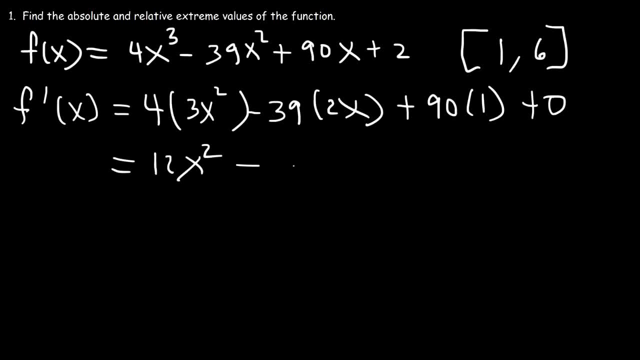 4 times 3, which is 12.. So that's 12x squared 39 times 2 is 78.. And then plus 90. So let's set the first derivative equal to 0.. Now notice that all of the coefficients are even. 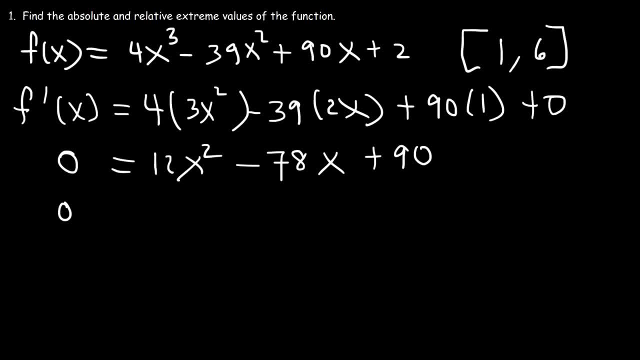 So we can divide everything by 2.. If we do so, if we divide both sides by 2, on the left, 0 divided by 2 is 0.. On the right, half of 12 is 6.. Half of 78 is 39.. 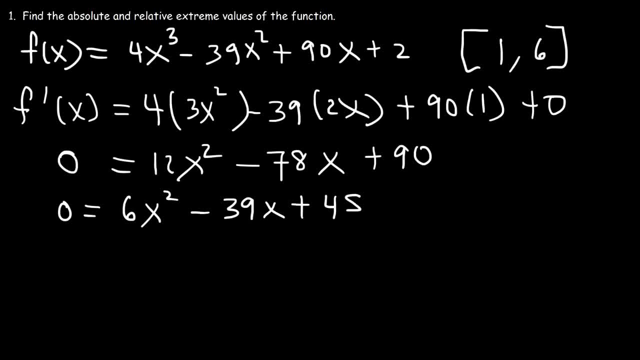 And half of 90 is 45. Now 6,, 39, and 45,. they are divisible by 3. So let's divide everything by 3.. So this is going to be 0. And then 6 divided by 3 is 2.. 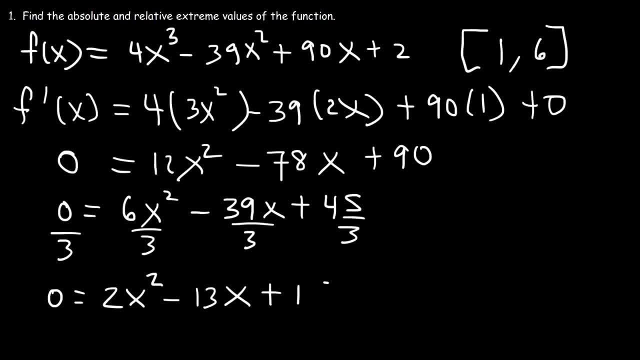 39 divided by 3 is 13.. 45 divided by 3 is 15.. So now let's factor the expression that we have. By the way, if you want the first derivative in its factored form, we divided everything by 6.. 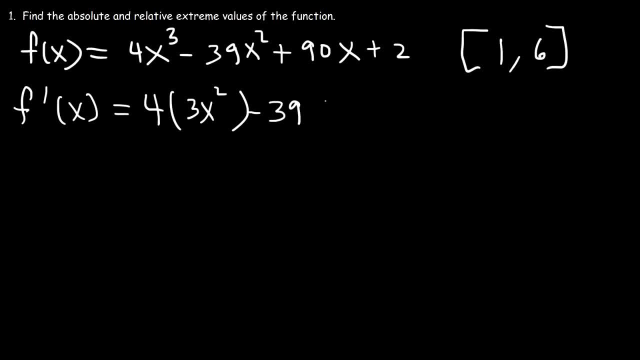 And the derivative of x squared is 2x. The derivative of x is 1. And the derivative of a constant is 0.. So f prime of x is going to equal 4 times 3,, which is 12.. So that's 12x squared. 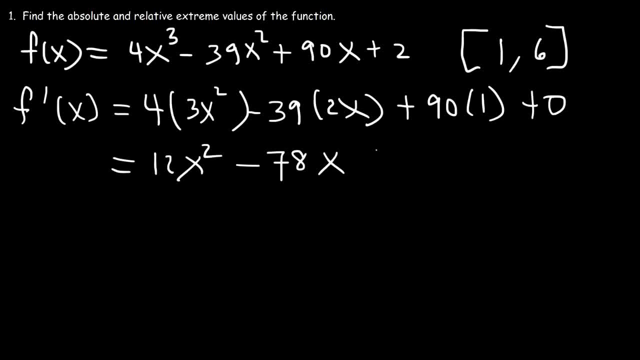 39 times 2 is 78.. And then plus 90. So let's set the first derivative equal to 0.. Now notice that all of the coefficients are even, So we can divide everything by 2.. If we do so, if we divide both sides by 2, on the left, 0 divided by 2 is 0.. 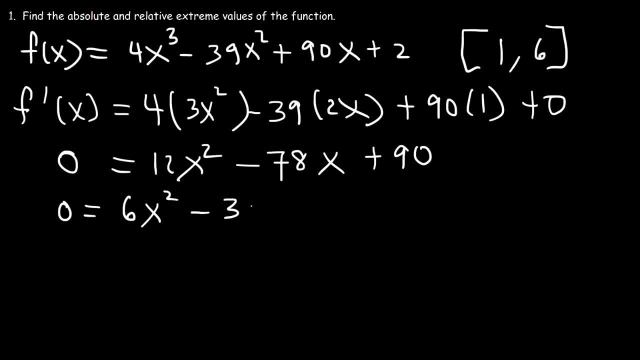 On the right, half of 12 is 6.. Half of 78 is 39. And half of 90 is 45. Now 6,, 39, and 45,- they are divisible by 3.. So let's divide everything by 3.. 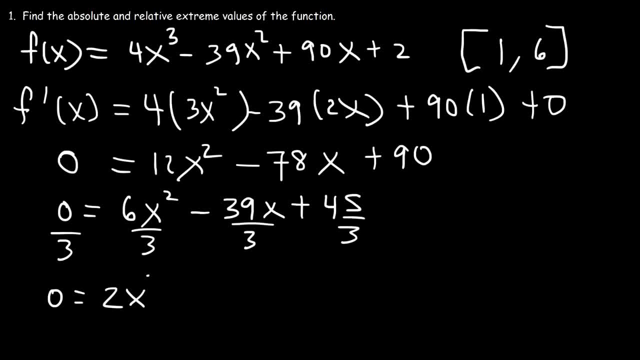 So this is going to be 0. And then 6 divided by 3 is 2.. 39 divided by 3 is 13.. 45 divided by 3 is 15.. So now let's factor the expression that we have. 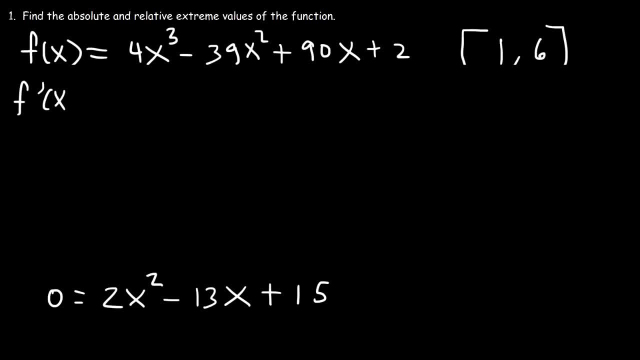 By the way, it's not always easy. By the way, if you want the first derivative in its factored form, we divided everything by 6. So you can write it like this if you want to. So how can we factor 2x squared minus 13x plus 15?? 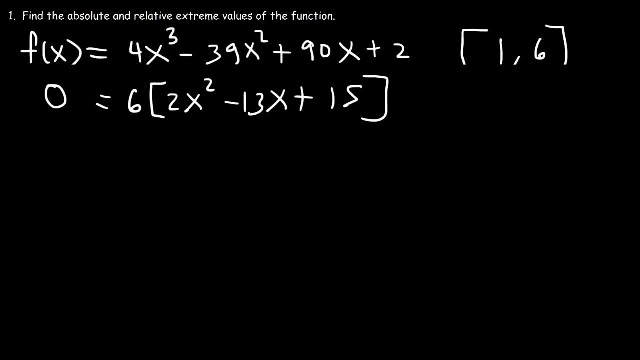 How can we do that? So first, we need to multiply the leading coefficient. We need to multiply the leading coefficient by the constant term. You need to do that any time. this number is anything but 1.. 2 times 15 is 30.. 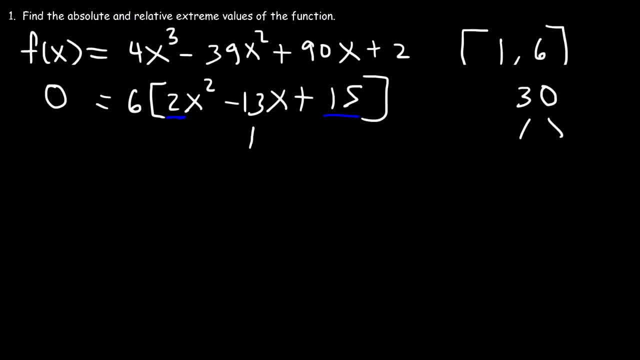 Now we need to find two numbers that multiply to 30 but add to the middle coefficient of negative 13.. So this is going to be 10 and 3,, both of which are negative, Because negative 10 times negative 3 is positive 30.. 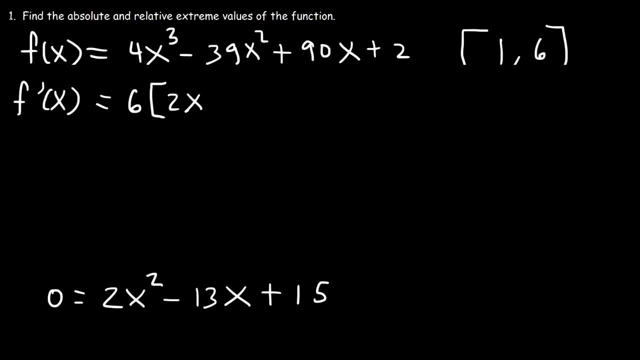 So you can write it like this if you want to. So how can we factor 2x squared minus 13x plus 15? How can we do that? So first we need to multiply the leading coefficient by the constant term. You need to do that any time this number is anything but 1.. 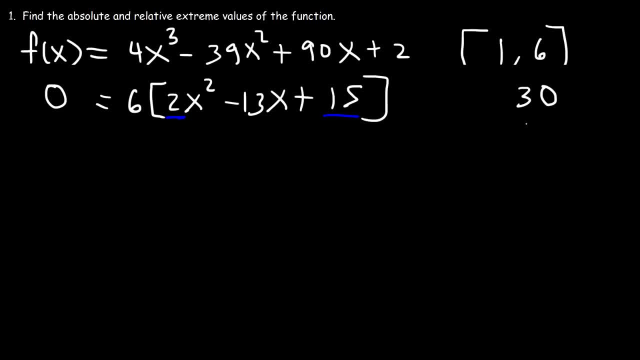 2 times 15 is 30. Now we need to find two numbers that multiply to 30 but add to the middle coefficient of negative 13.. So this is going to be 10 and 3, both of which are negative Because negative 10 times negative, 3 is positive 30. 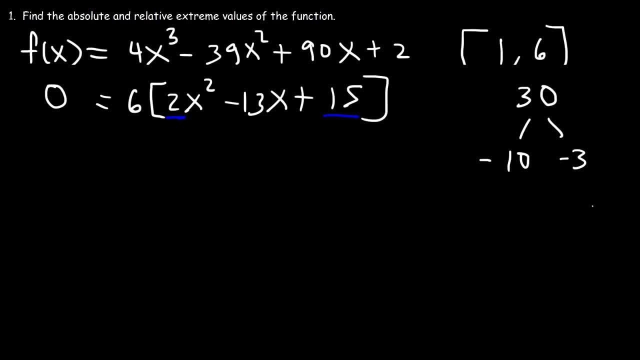 But negative 10 plus negative 3 adds up to negative 13.. So what we're going to do is replace the middle term negative 13x with negative 10x minus 3x, And then we need to factor by grouping. 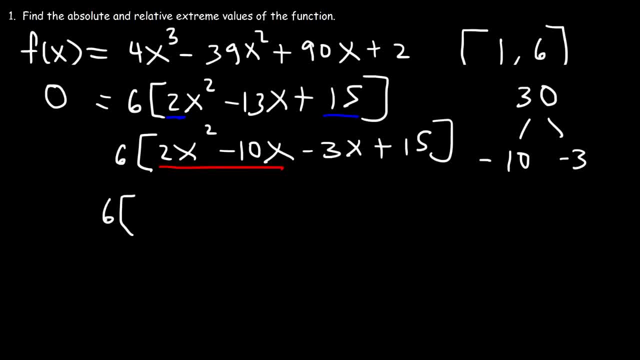 So take out the GCF. in the first two terms, The greatest common factor is 2x. 2x squared divided by 2x is x Negative. 10x divided by 2x is negative 5.. And the last two terms take out the greatest common factor, which is going to be negative: 3.. 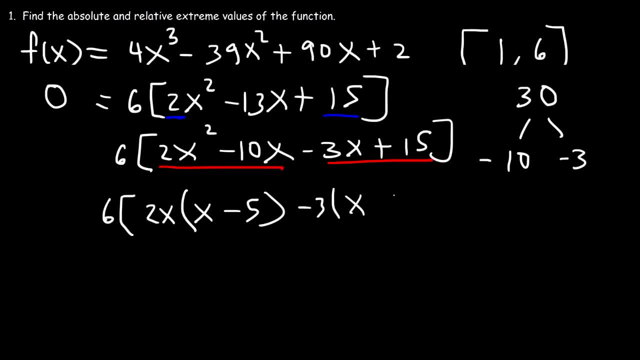 Negative: 3x divided by negative, 3 is x. Positive: 15 divided by negative, 3 is negative, 5.. So now we need to factor out x minus 5.. So this term divided by x minus 5, these two will cancel, leaving behind 2x. 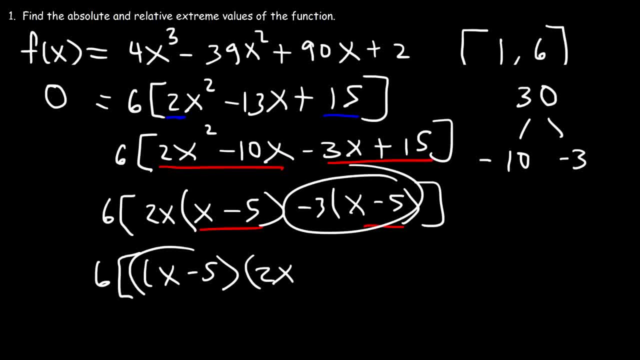 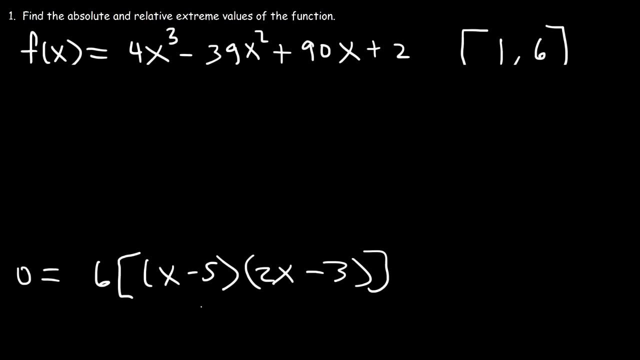 And if we take this term divided by x minus 5, these will cancel, giving us negative 3.. So this is the first derivative in its factored form. Now we need to set each factor equal to 0. So if we set x minus 5 equal to 0,, 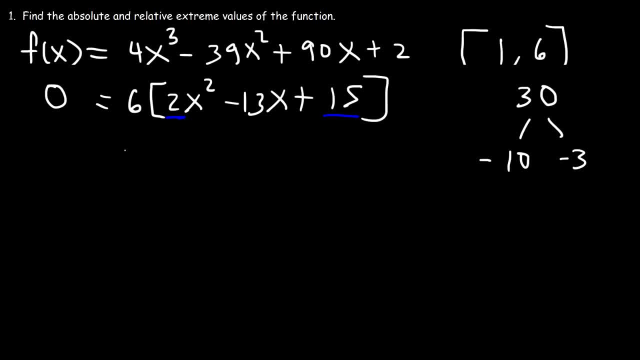 But negative 10 plus negative 3 adds up to negative 13.. So what we're going to do is replace the middle term negative 13x with negative 10x minus 3x, And then we need to factor by grouping. 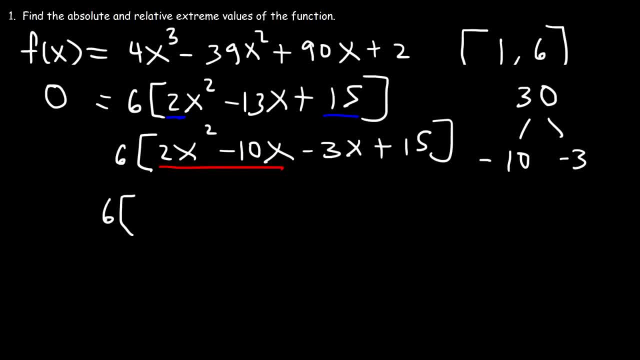 So take out the GCF. in the first two terms, The greatest common factor is 2x. 2x squared divided by 2x is x Negative. 10x divided by 2x is negative 5.. And the last two terms take out the greatest common factor, which is going to be negative: 3.. 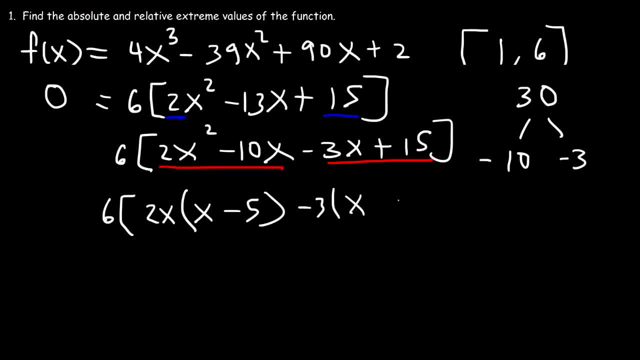 Negative: 3x divided by negative, 3 is x. Positive: 15 divided by negative, 3 is negative, 5.. So now we need to factor out x minus 5.. So this term divided by x minus 5, these two will cancel, leaving behind 2x. 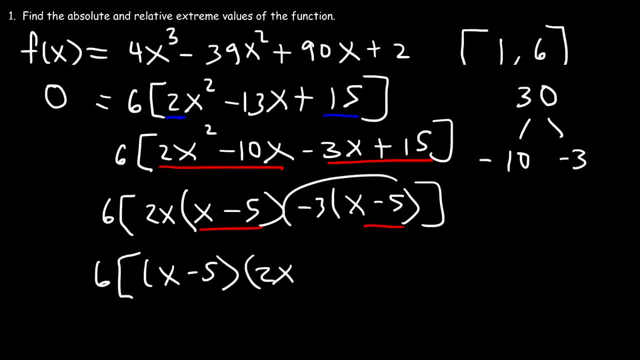 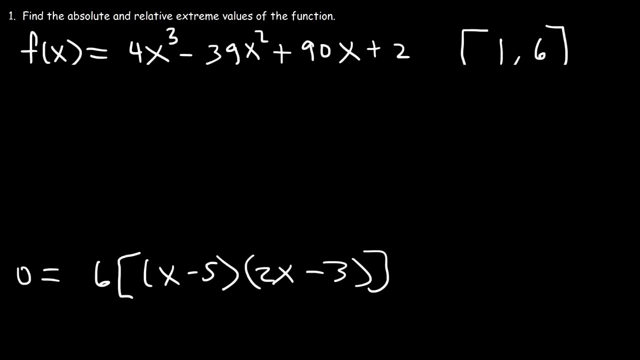 And if we take this term divided by x minus 5, these will cancel, giving us negative 3.. So this is the first derivative in its factored form. Now we need to set each factor equal to 0. So if we set x minus 5 equal to 0 and add 5 to both sides, 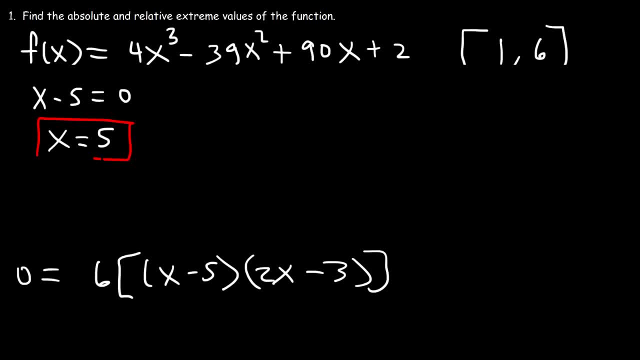 this is the first critical number. x is equal to 5.. And then let's set the other factor, 2x minus 3, equal to 0. So add 3 to both sides and then divide by 2.. So the second critical point is 3 over 2.. 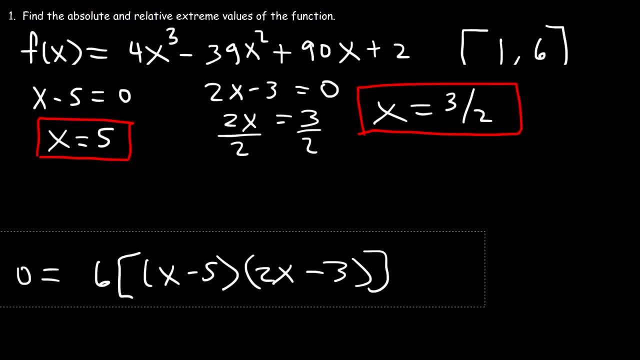 So now we need to make a sign chart to determine which of those critical points represent the relative maximum and which one is the relative minimum. 3 over 2 comes before 5.. So let's pick a number that's greater than 5.. 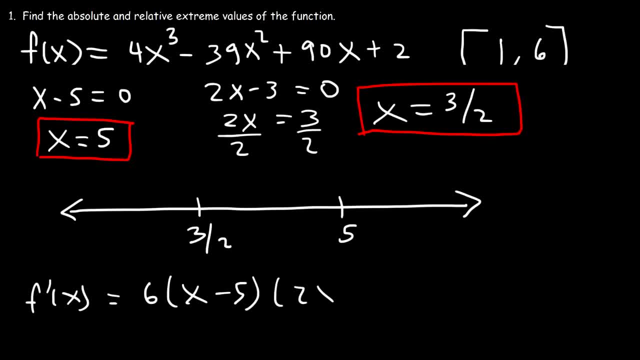 And I need to rewrite this expression. So let's try 6.. If we plug in 6, will the first derivative be positive or negative? 6 minus 5 is positive. 2 times 6 minus 3 is also positive. 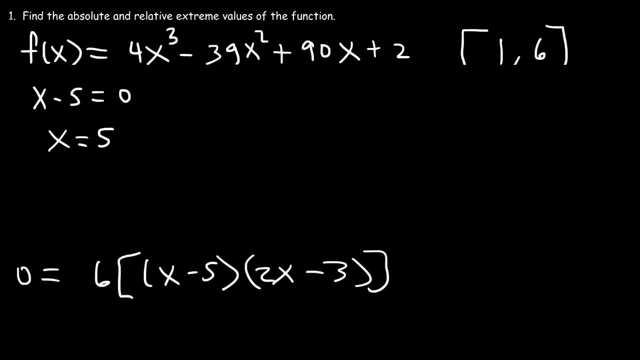 and add 5 to both sides. this is the first critical number. x is equal to 5.. And then let's set the other factor, 2x minus 3, equal to 0. So add 3 to both sides and then divide by 2.. 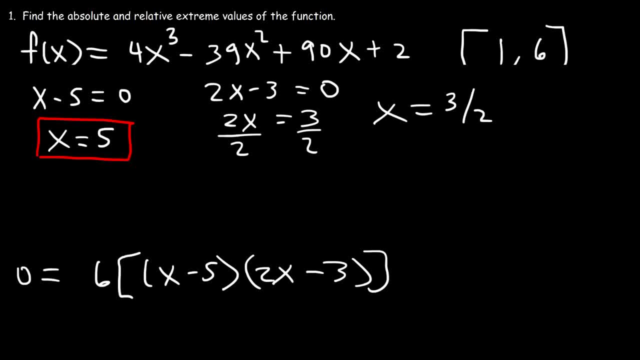 So the second critical point is 3 over 2.. So now we need to make a sign chart to determine which of those critical points represent the relative maximum and which one is the relative minimum. 3 over 2 comes before 5.. 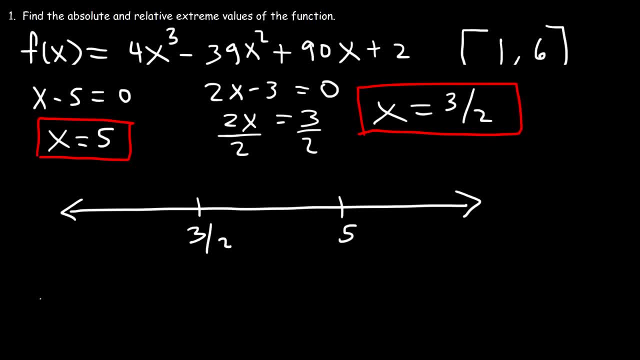 So let's pick a number that's greater than 5.. And I need to rewrite this expression, So let's try 6.. If we plug in 6, will the first derivative be positive or negative? 6 minus 5 is positive. 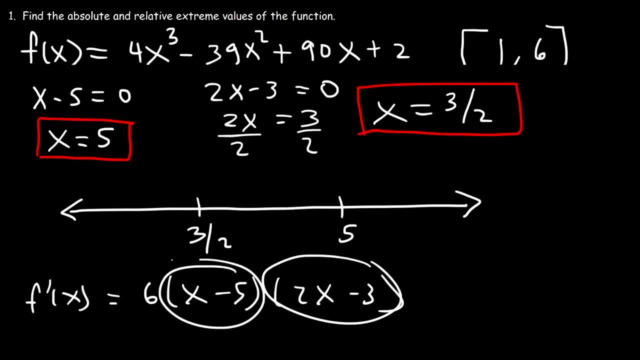 2 times 6 minus 3 is also positive. So if we multiply two positive numbers, this will give us a positive result. Now notice that for each factor we have an odd exponent. That means the signs will change across each critical number. 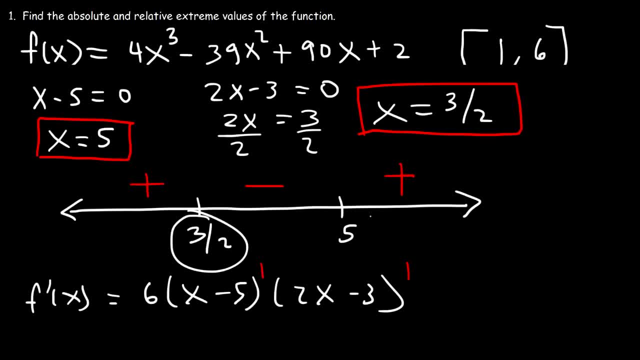 So if you pick a number between 1.5 and 5, it's going to be negative. So let's try 2.. 2 times 2 minus 3. That's positive. That's equal to a positive 1.. 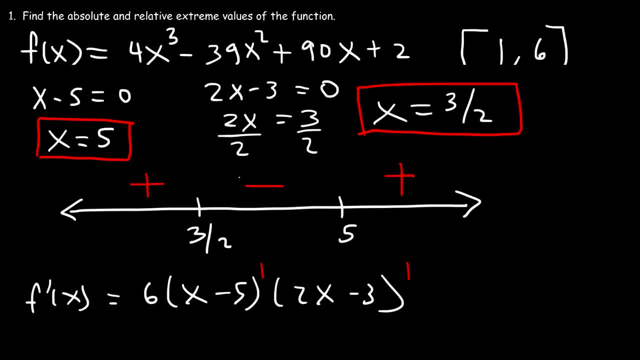 2 minus 5 is negative. A negative number times a positive number will give us a negative result, And if we pick something that's less than 3 over 2, like 0, that will be positive. 0 minus 5 is negative. 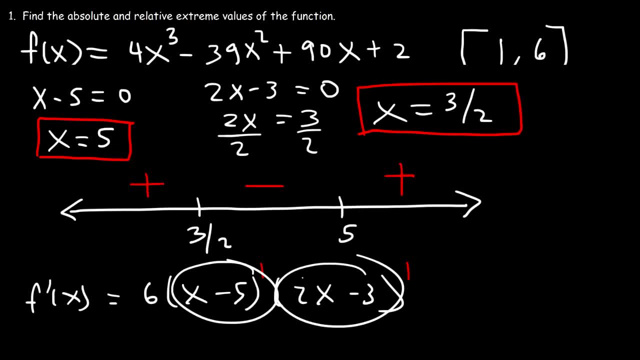 2 times 0 minus 3 is also negative. If you multiply two negative numbers, that will give you a positive result. Now, which of these critical numbers represents a maximum and which one is a minimum? Well, let's focus on 3 over 2.. 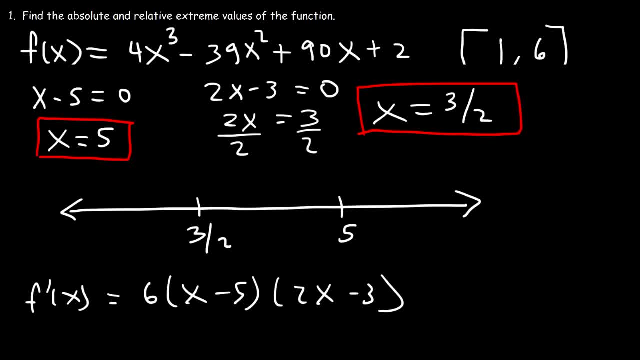 So if we multiply two positive numbers, this will give us a positive result. Now notice that for each factor we have an odd exponent. That means the signs will change across each critical number. So if you pick a number between 1.5 and 5, it's going to be negative. 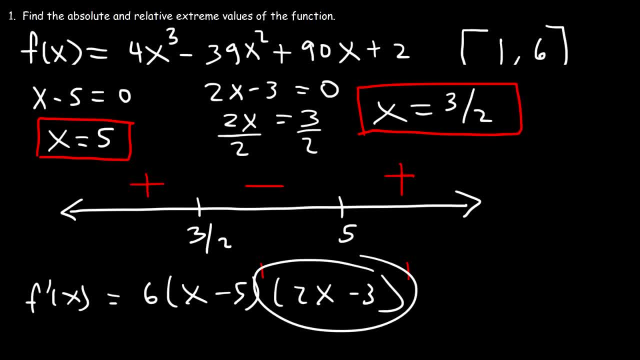 So let's try: 2. 2 times 2 minus 3, that's positive, That's equal to positive. 1. 2 minus 5 is negative. A negative number times a positive number will give us a negative result. And if we pick something that's less than 3 over 2, like 0, that will be positive. 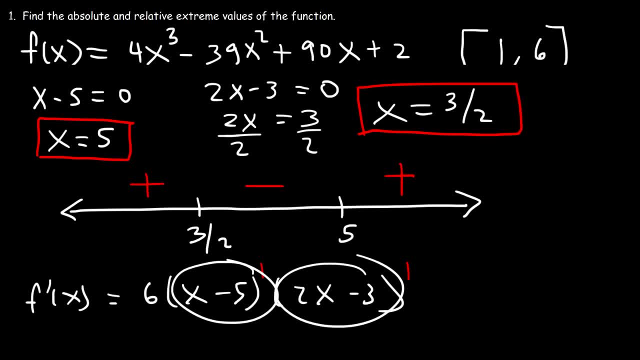 0 minus 5 is negative. 2 times 0 minus 3 is also negative. If you multiply two negative numbers, that will give you a positive result. Now, which of these critical numbers represents a maximum and which one is a minimum? 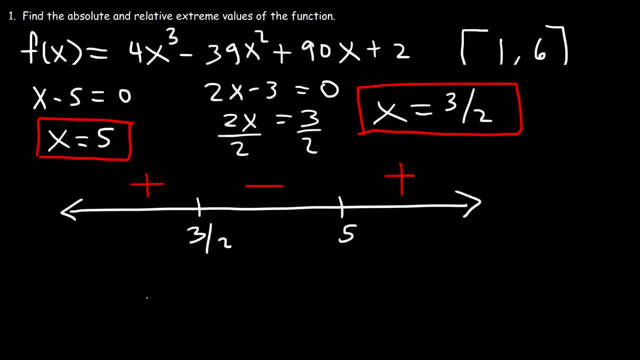 Well, let's focus on 3 over 2.. The function is increasing and then it's decreasing, So that represents a maximum. And for 5, it's decreasing first and then it's increasing, So that's a minimum. So now let's make a table. 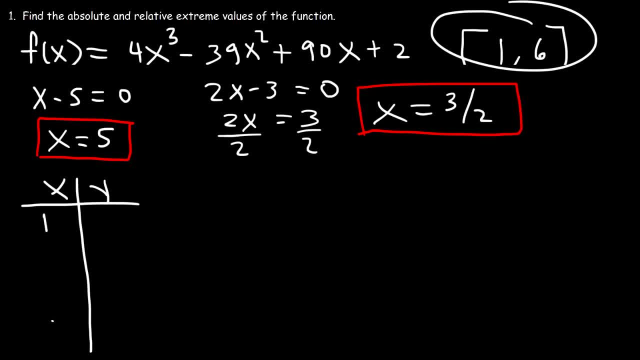 So let's put the endpoints So we have 1 and 6. And make sure that the critical numbers are in this interval. If they're not, you can't use them. So 3 over 2 is 1.5.. 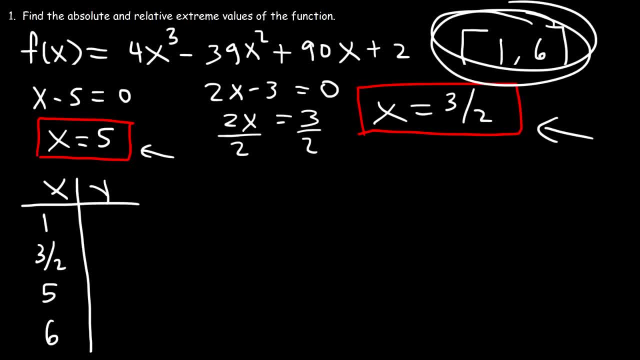 That's between 1 and 6. And so is 5.. Now let's identify the y values for each of the x values. So let's start with 1.. This is going to be 4 minus 39 plus 90 plus 2.. 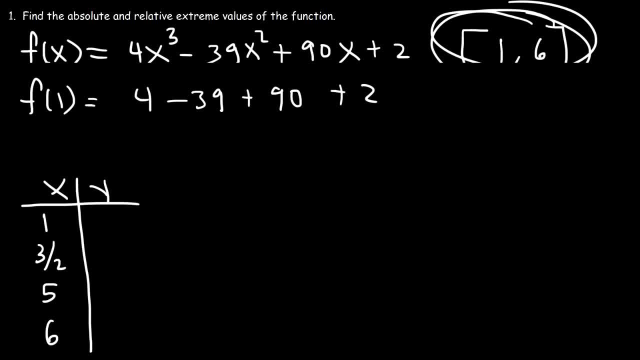 And I'm going to use a calculator for this one. So I got 57 when x is 1.. Now when x is 3 over 2, or 1.5, this is going to be 4 times 1.5 to the third power. 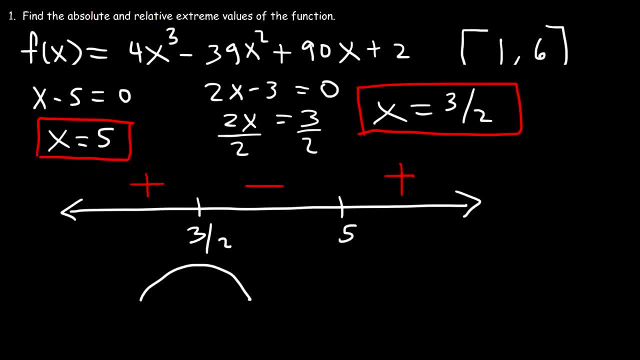 The function is increasing and then it's decreasing, So that represents a maximum. And for 5, it's decreasing first and then it's increasing, So that's a minimum. So now let's make a table. So now let's make a table. 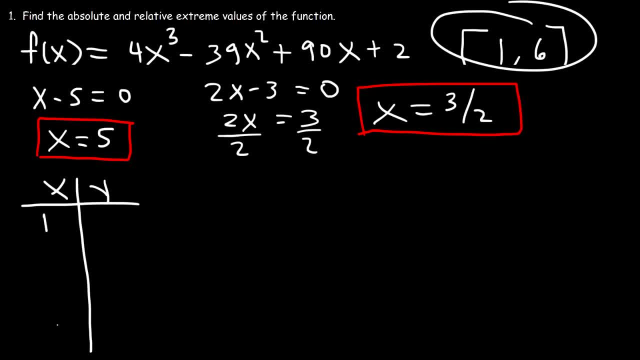 So let's put the endpoints So we have 1 and 6. And make sure that the critical numbers are in this interval. If they're not, you can't use them. So 3 over 2 is 1.5.. 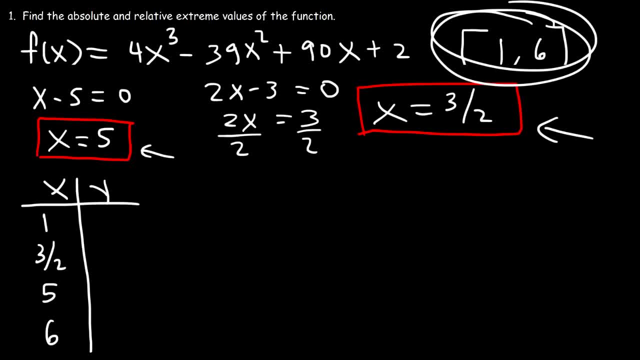 That's between 1 and 6. And so is 5.. Now let's identify the y values for each of the x values. So let's start with 1.. This is going to be 4 minus 39 plus 90 plus 2.. 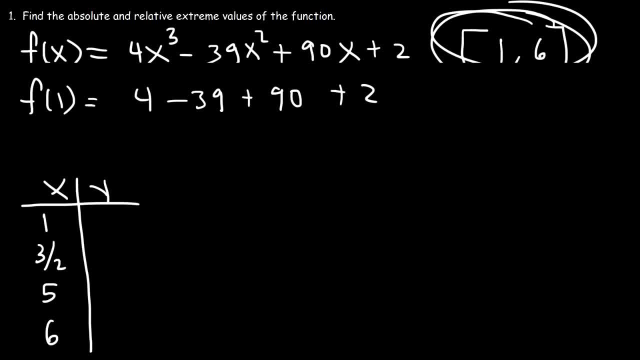 And I'm going to use a calculator for this one. So I got 57 when x is 1.. Now when x is 3 over 2, or 1.5,, this is going to be 4 times 1.5 to the third power, minus 39 times 1.5 squared plus 90 times 1.5 plus 2.. 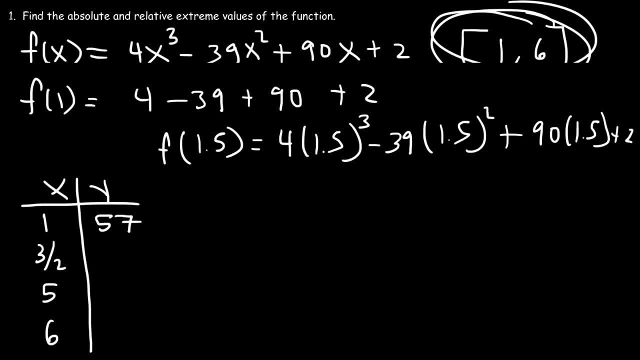 So hopefully you're allowed to use calculators on a test, Because this will take a while. We could do it without a calculator, but I'm not going to do it in this video, So I got as a decimal 62.75.. 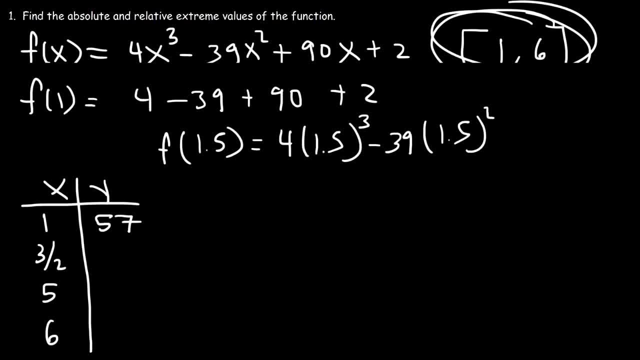 minus 39 times 1.5 squared plus 90 times 1.5 plus 2.. So hopefully you're allowed to use calculators on a test, Because this will take a while. We could do it without a calculator, but I'm not going to do it in this video. 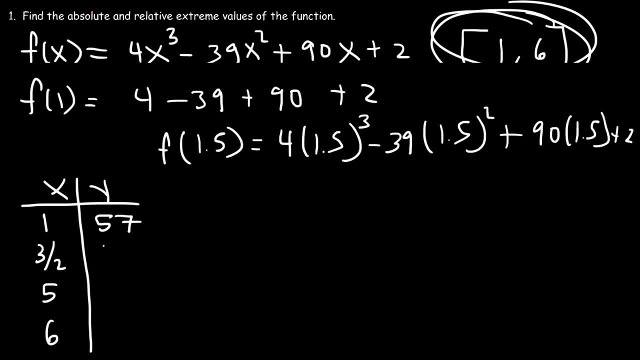 So I got, as a decimal, 62.75.. Now, for f of 5,- I'm just going to type it in- I got negative 23.. And then for f of 6, I got 2.. Now, which of these points represent the absolute maximum? 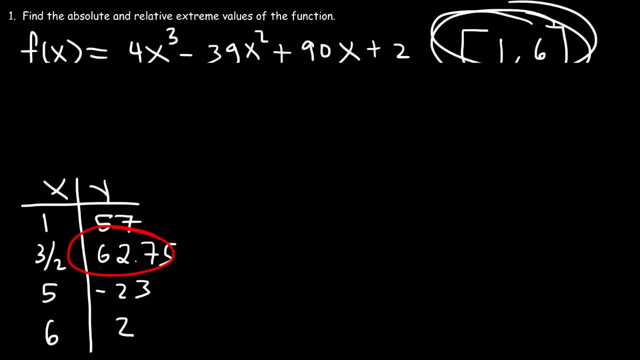 In this interval, 62.75 is the highest value, So this is the absolute maximum. What about the absolute minimum? Negative 23 is the lowest y value listed. So 5 comma negative 23,. that's the absolute minimum. So the absolute minimum of the function is located at x equals 5.. 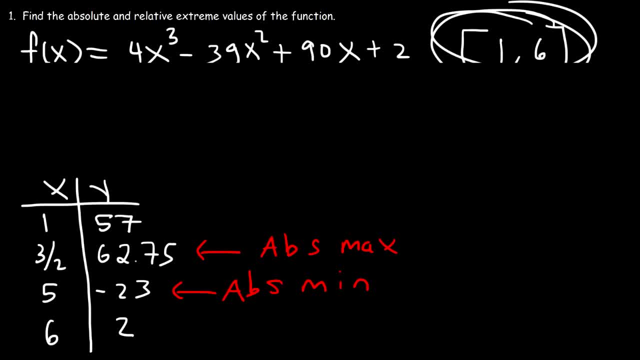 But the absolute minimum value that represents the y coordinate. the value is negative 23. So typically the location is associated with the x coordinate, but the value is associated with the y coordinate. Now we said that 3 over 2 was also the relative maximum. 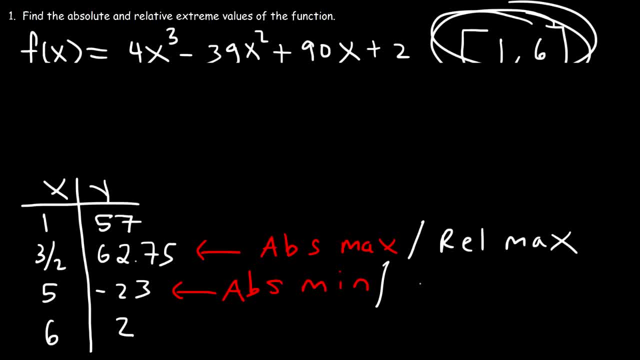 It was a critical number And 5 was a relative minimum. So sometimes the endpoints they may be an absolute max or an absolute minimum. You don't know. You have to check it Other times. the absolute max can be the relative max. 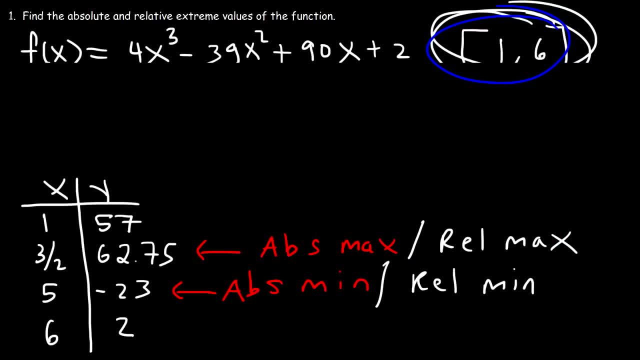 And the absolute minimum can be the relative minimum. So you need to make the table, Make sure you put the endpoints of the closed interval and the critical points in the table and then just compare the y values. So that's it for this video. 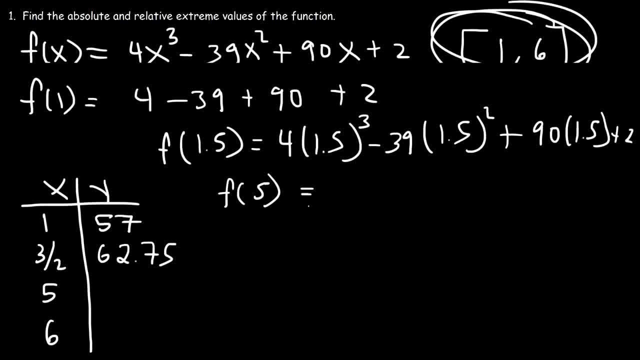 Now for f of 5,- I'm just going to type it in- I got negative 23.. And then for f of 6, I got 2.. Now, which of these points represent the absolute maximum In this interval? 62.75 is the highest value. 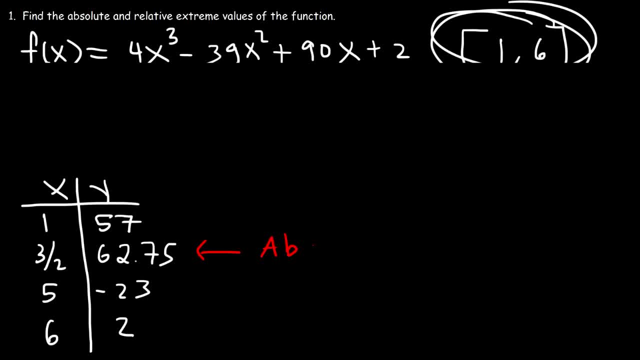 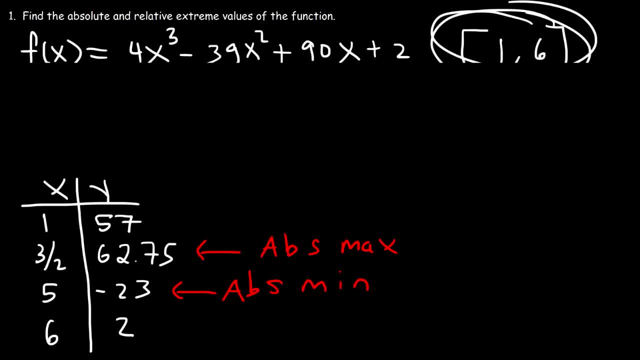 So the absolute minimum of the function is located at x equals 5.. But the absolute minimum value that represents the y coordinate, the value, is negative 23.. So typically the location is associated with the x coordinate, but the value is associated with the y coordinate. 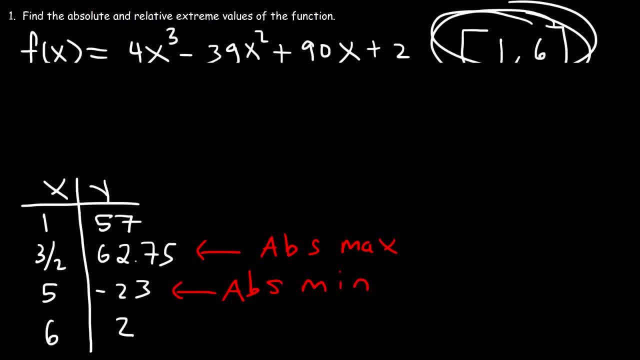 Now we said that 3 over 2 was also the relative maximum. It was a critical number And 5 was a relative minimum. So sometimes the endpoints they may be an absolute max or an absolute minimum. You don't know. You have to check it. 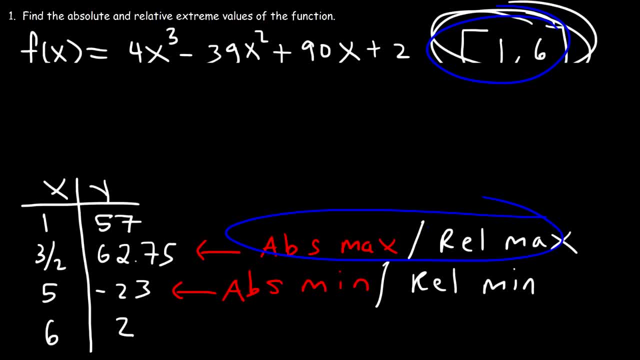 Other times the absolute max can be the relative max And the absolute minimum can be the relative minimum. So you need to make the table. Make sure you put the endpoints of the closed interval and the critical points in the table and then just compare the y values. 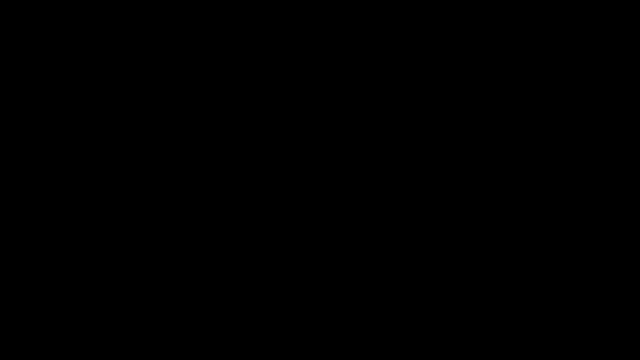 So that's it for this video. Thank you.